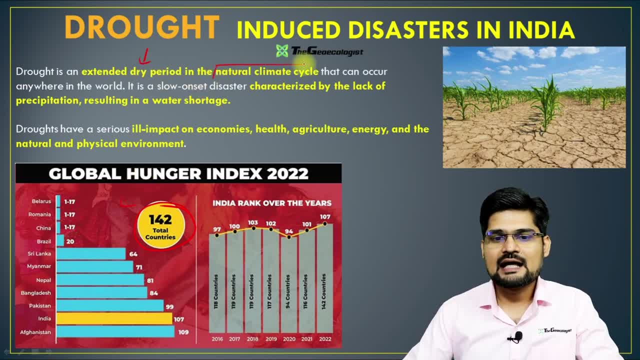 So what is drought? It's basically an extended period of dryness in the natural climate cycle and largely characterized by the lack of precipitation of various forms. So you'll observe, the resultant is water shortage. And with water, what is associated? Agriculture. 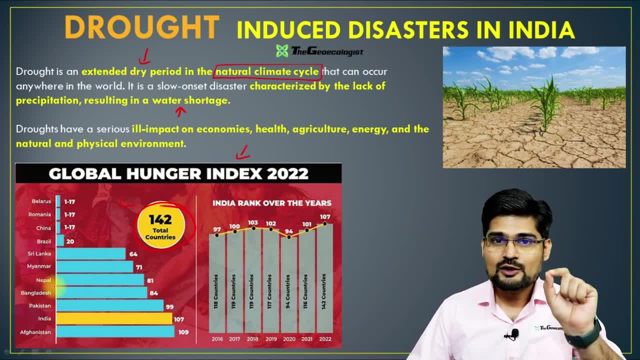 food security. So you observe here hunger index, isn't it? So a lot of it has to do with drought situation across the world and India. So impacts on economies, health, agriculture, energy- everywhere in the ecosystem you'll find. 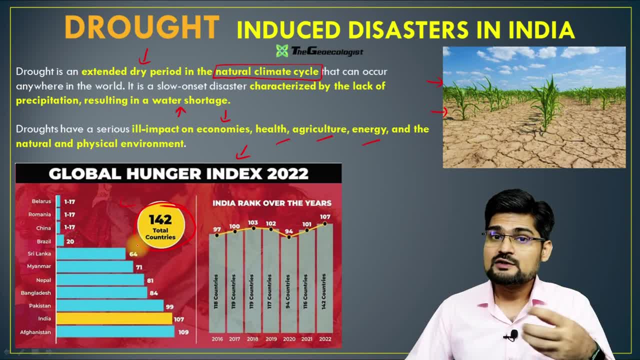 That this drought has an impact And remember the world is already food insecure. We keep talking about it as the population is growing and right from Malthusian theory of population to the modern theories, the economic theories, we have been learning about it. So what you? 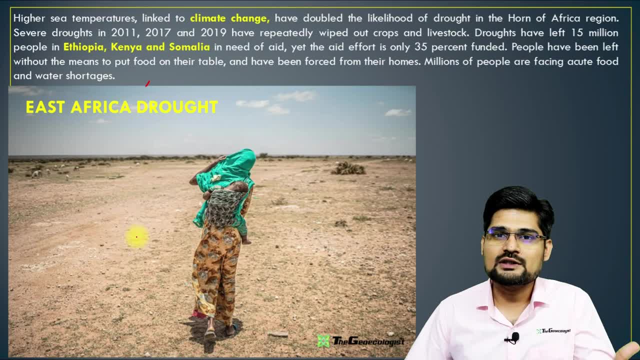 observe there is an incidence of extreme drought across the world. One of the prime examples that we also discussed in the earlier lectures is this: East Africa drought. Do you realize the areas in Ethiopia, Kenya, Somalia? Look into this persistent drought since last decade. 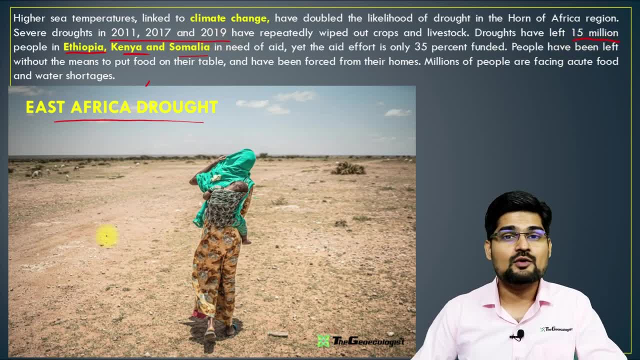 And how many people- 15 million people or more- have been affected already. So this is the ground reality. That's why it's very important to understand the nuances of drought, the various aspects of drought, its classification. So look into the Indian scenario Now. if you 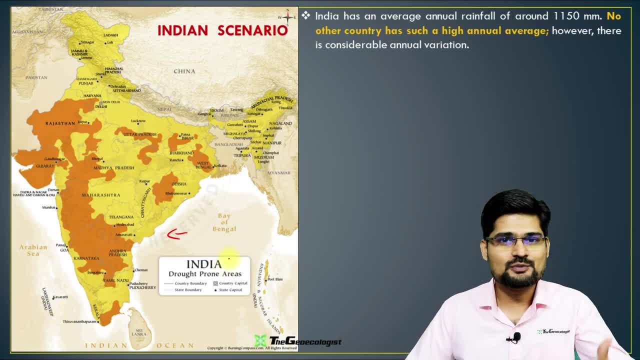 observe the physiography of India. if you know the physical geography, the geomorphology of India, you know that it's a very uneven and diverse country in all the ways. So what you observe here, that floods and drought are simultaneous in India. So some areas. 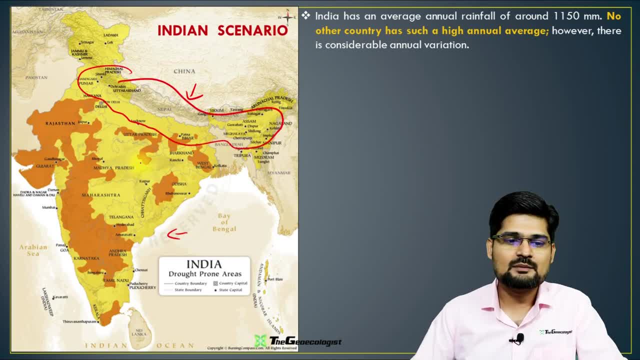 in today's India are affected by flood, while some are facing acute shortage of water. This is unevenness, although our annual average is good, 1150 millimetres. But looking at that figure, you may not understand the reality on the ground. So if you observe this map, 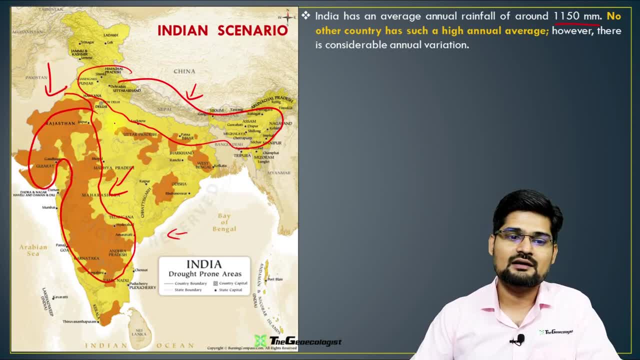 this brown patch across the map, considerable area of India right. You observe these pockets. everywhere you have acute shortage of water and obviously these places are where agriculture week. So what do you observe? Food insecurity alongside drought, And that's where vulnerabilities. 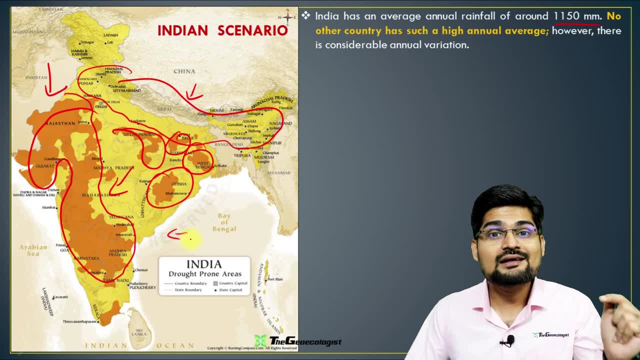 arise, And that's why we're talking about drought-induced disasters. If people are not having enough food to eat, they're not able to survive. that's definitely creating a vulnerable situation, disastrous situation. So if you observe here, more than 80% of the total rainfall that we 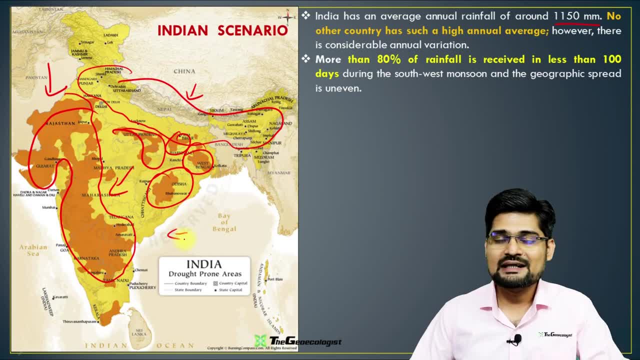 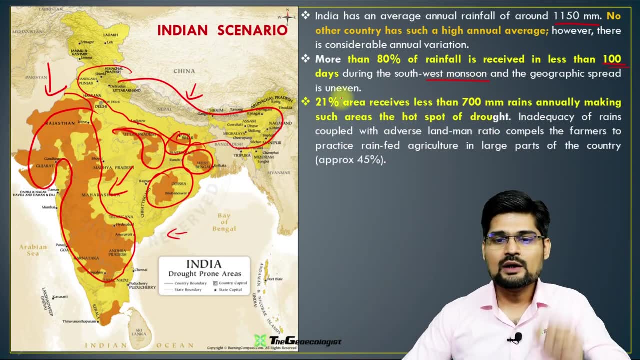 receive during monsoon season is concentrated in only 3 months, 100 days of rainfall, And that's through southwest monsoon, as we know. So what's happening here? 21% area receives less than 700 millimeter rainfall annually, making it a huge hotspot for drought. You can observe in the map: 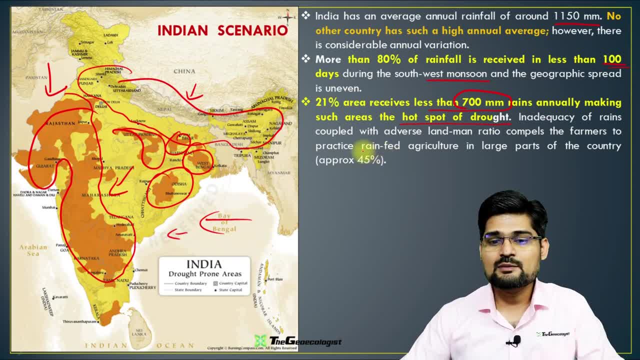 itself, isn't it? So what you observe? we have maximum rain-fed agriculture in large parts of the country, approximately 45%. So we are all monsoon-dependent country, monsoon-dependent economy, And if it fails certain years, if there is an El Nino year where you have most probable, 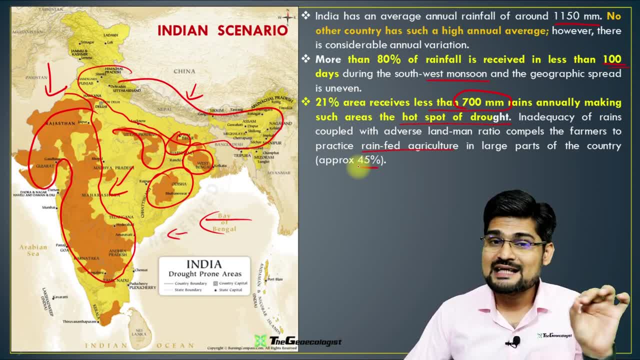 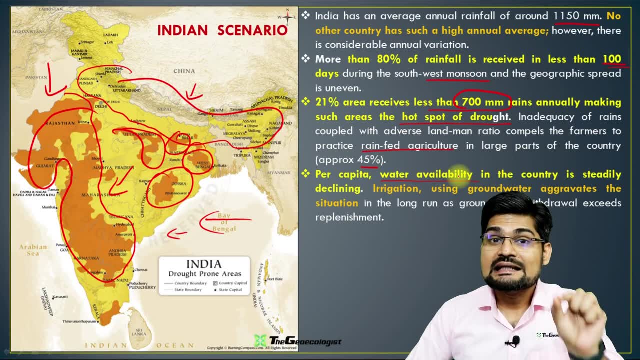 drought situation. it's not going to happen. So what's happening here? We're talking about a huge situation. it's a disastrous situation. So what you observe here: per capita water availability in the country is also declining steadily and it's a huge issue now. So what's? 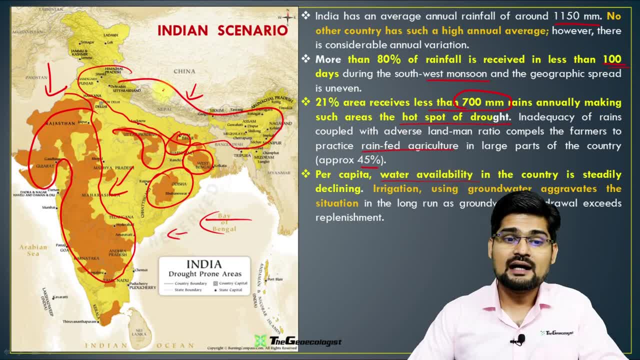 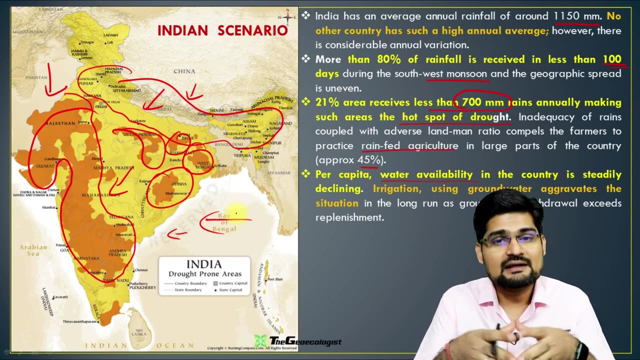 happening Per capita water availability. So you mean that one person is not having enough water per day as per the basic consumption rate And on the top irrigation? So do you realize that all our irrigation is dependent on the rainfall that we have, And in certain areas we also have canal. 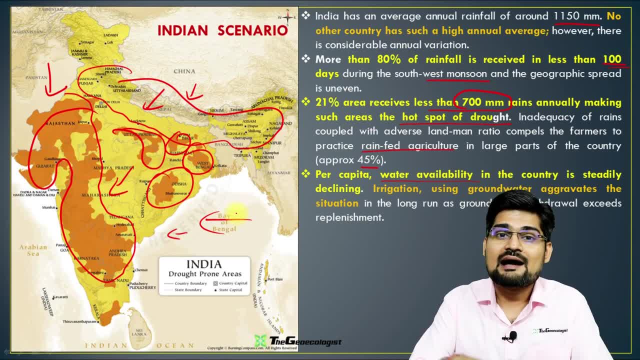 irrigation, But, majorly, we are dependent on the groundwater, And the groundwater will only be recharged if you have enough rainfall. So there is a vicious cycle out here. So this is what we observe is that groundwater is not being replenished as it is being consumed. And also remember, 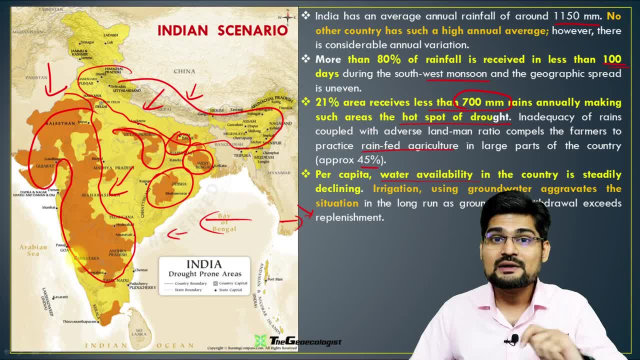 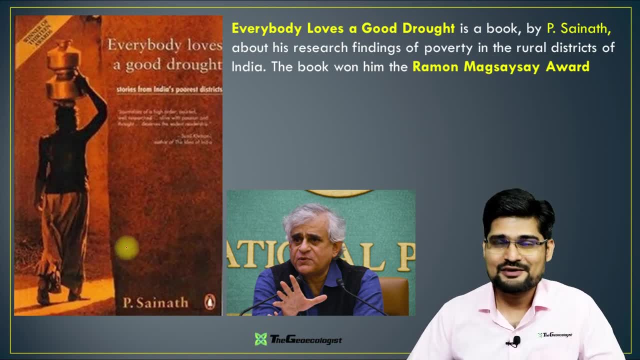 now. we are the most populous country in the world, So requirement is going to be higher day by day, And that's a huge situation. Now, looking into this particular book that I'm referring you here to, this is a book that you can definitely read for all the aspirants, especially for people who love 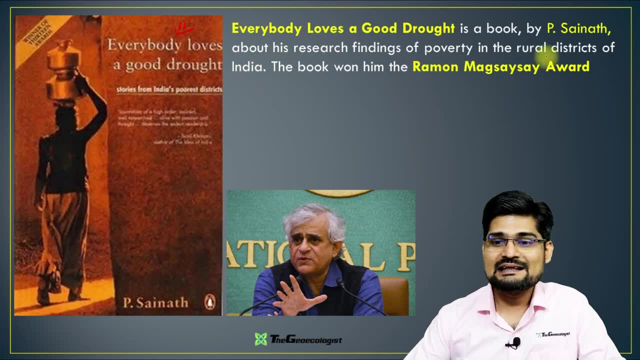 to read different perspectives of drought. So this is one book by P Sainath. Remember this author, P Sainath, is a Raman Magasase Award winner And he wrote this book called Everybody Loves a Good Drought. And you remember? this is a satire, this is a comment on our system. So what's happening? 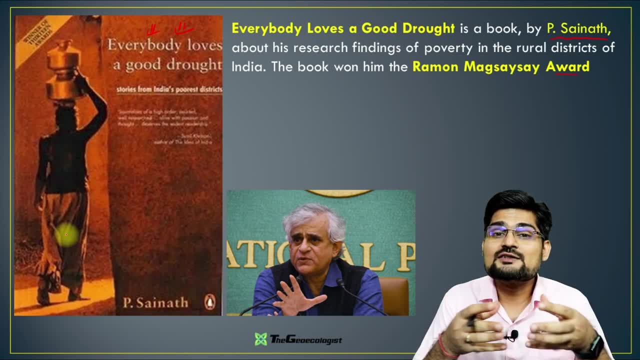 Why people love drought in our country or, for that matter, floods? because people are so vulnerable, so poor, that they cannot earn their living from other means. So they wait for government to do a drought or flood and then they get the relief funds. And that's how you see the observe this. 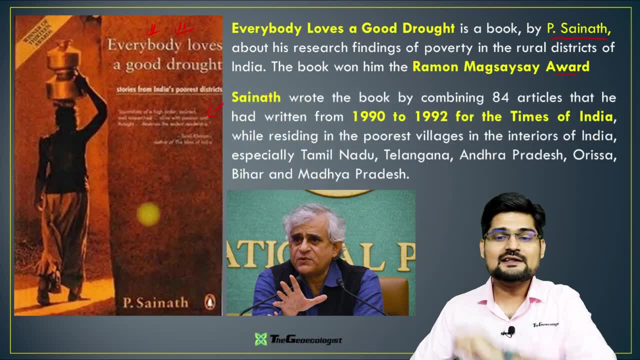 particular book So you can see India's poorest districts. So this book, P Sainath has talked about many things that in 90s he observed. for Times of India he wrote, and in Tamil Nadu, Telangana, Andhra Pradesh, Odisha, Bihar, MP, all these states where drought situation is there. 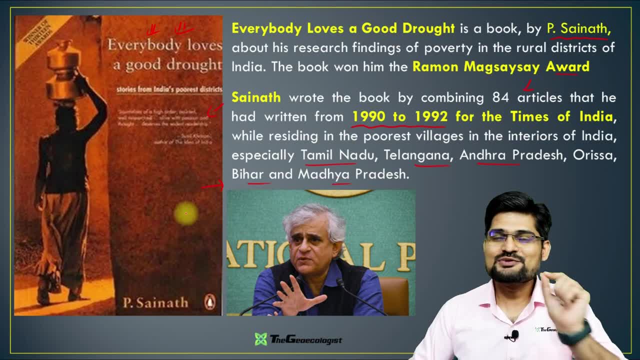 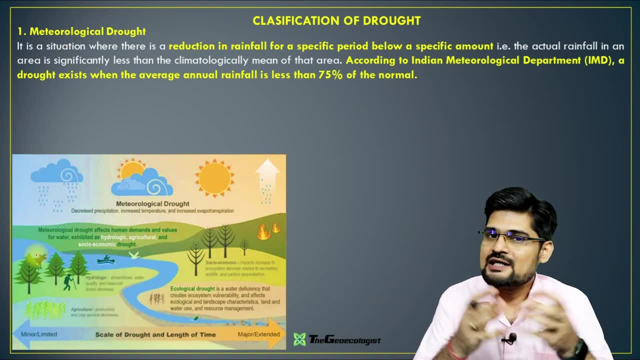 and how people react to these situations right. So this is one of the read. Now let's continue on our topic, And first thing that we should know is classification of drought. So I'm sure you have seen this drought classification earlier as well. 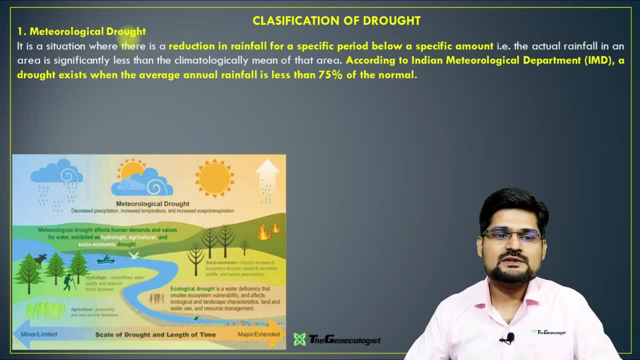 So meteorological drought, agricultural drought, right? So what you observe is the first kind of drought, that is, meteorological drought. Now it's meteorology coming to the picture, climate science coming to the picture. So basic idea is reduction of rainfall for 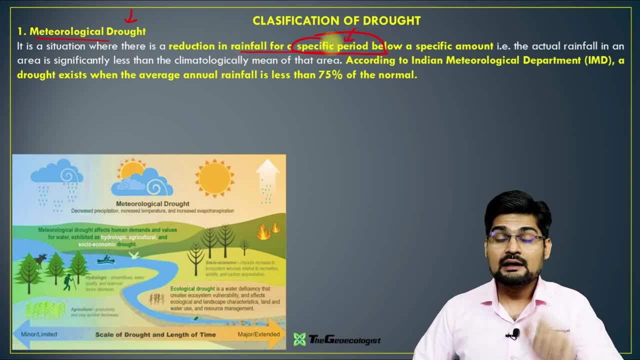 specific period. Now, this is specific time period in a specific amount. So what you observe, Indian meteorological department, what does it say? So, according to IMD, what you observe, drought exists when average annual rainfall is less than 75% the normal. So if average is below, 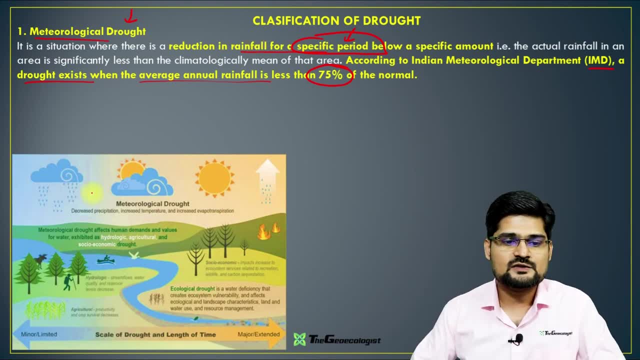 75, then it is a meteorological drought And you can observe this meteorological drought image as well. You can pause the video and you can draw this diagram for yourself as well. So look into the situation. The cause is lean monsoon- definitely a huge role to play- and below average. 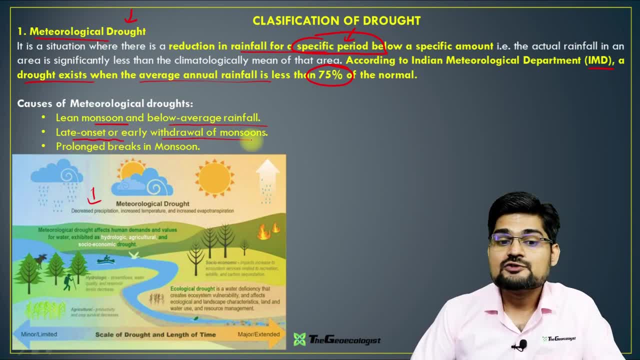 rainfall, Also late onset or early withdrawal of monsoon. So monsoon is not just one factor. Remember, monsoon is not just one factor, it's also a factor. So monsoon is not just one factor. Remember, monsoon is not just one factor. So monsoon is not just one factor. So monsoon is not just one factor. 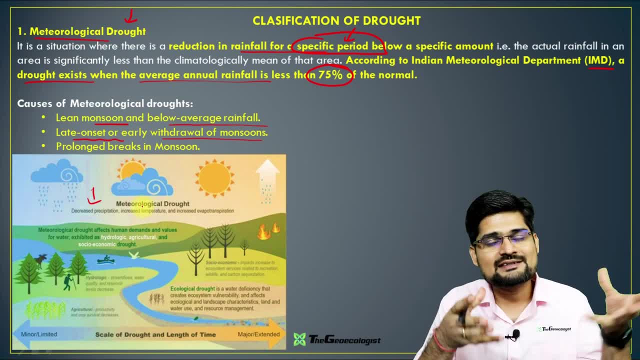 Sometimes it's disturbed because of Western disturbance, because of local anomaly, because of El Nino, La Nina or Indian Ocean Dipole factors. So what you observe- this is a very important issue to look into- and prolonged breaks in monsoon. So this is the major cause for meteorological drought. 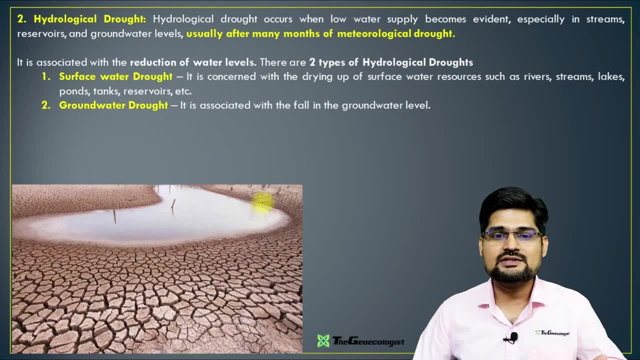 Now come to the other one, which is hydrological drought, hydrology, right, So surface and ground hydrology, if you see. So, months of meteorological drought leads to what It leads to: non-replenishing of underground water. So if our underground water is not being recharged on time, we'll have 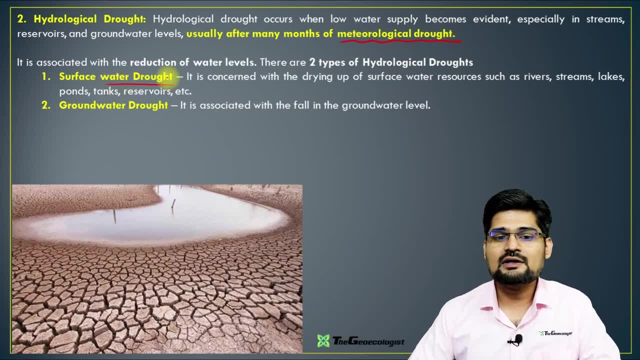 hydrological drought. So what you observe? surface water drought. it is concerned with drying up of surface water resources like rivers, streams, lakes- all of them have dried up right Pond tank reservoir. And what about groundwater? It's not being recharged, So you have the problems in. 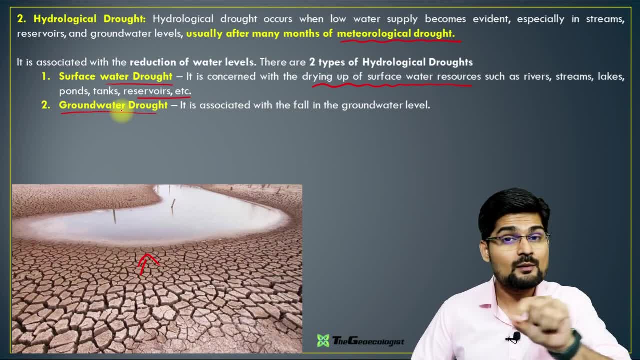 where you have bore wells and others, they all get dried up. This is a very common problem in North India these days. If you observe, in UP and Bihar and other places, a lot of wells, a lot of tube wells, are being dried up. So this is hydrological drought that you see And again. 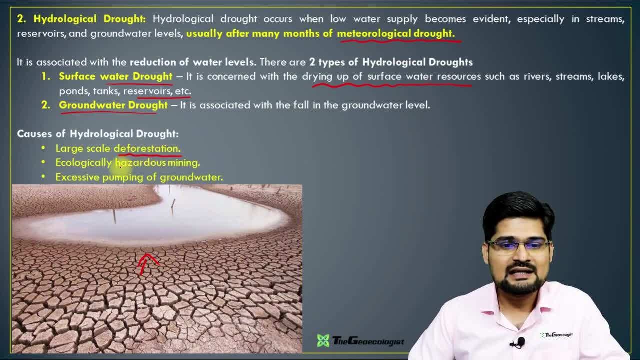 the reason here: large scale deforestation. then you have hazardous mining and also looking into the excessive pumping of groundwater. Remember groundwater. excessive pumping is not just for residential usage or industrial usage: 85% in India we use this groundwater for irrigation. 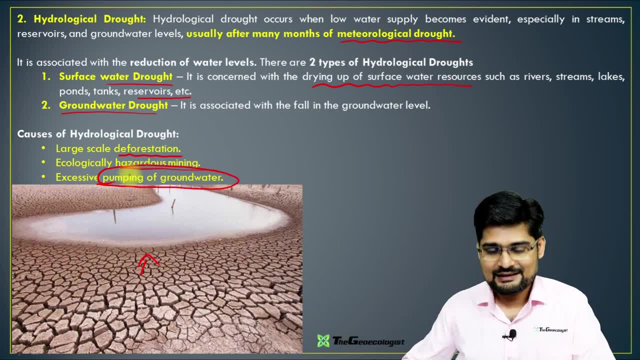 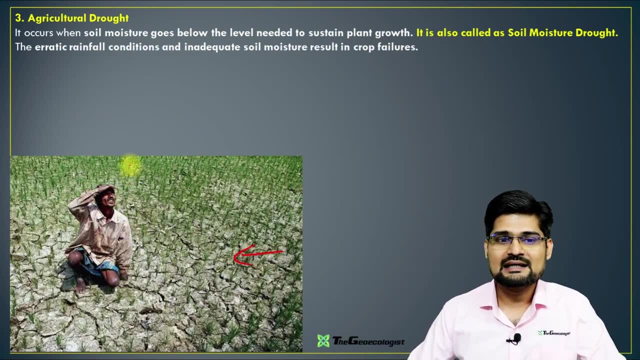 So that's why we say water harvesting has to be done right Now. look into the third category: agricultural drought. I'm sure you have seen these kind of pictures in newspaper and magazines. So what does it symbolize? It occurs when soil moisture- remember, soil moisture is very 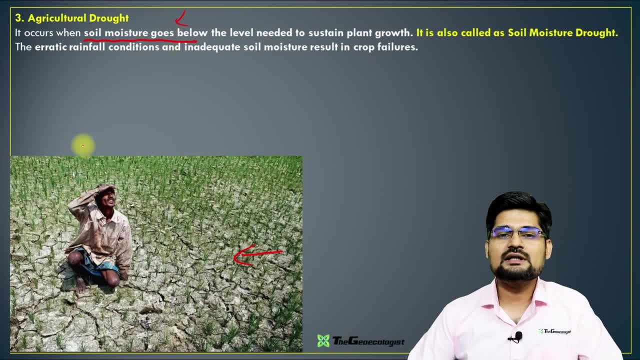 important, like soil carbon, right So soil moisture goes below the level of needed for the plant to survive, right? So every plant has a different level of moisture requirement, isn't it? So this is called soil moisture drought as well, or agricultural drought, where erratic rainfall 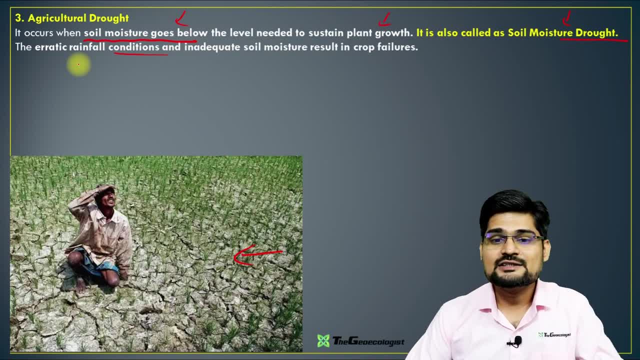 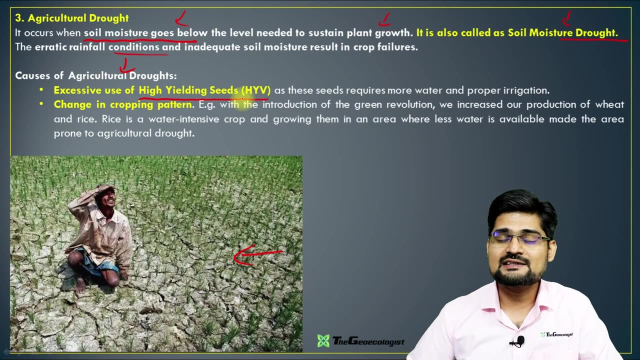 condition: hydrological drought can trigger this agricultural drought. And then the third category is crop failure. So this leads to crop failures. I'm sure you have seen in the news, because of crop failures there have been numerous cases of farmer suicides in our country. So what you observe here causes of these agricultural droughts. one of them is high yielding variety of seeds. Now remember HYV seeds came into existence in India, especially during Green Revolution. But do you realize one thing that it brought together was excessive irrigation is needed. So if you don't have proper irrigation, your crops will dry right. So change in cropping pattern as well. So because of the 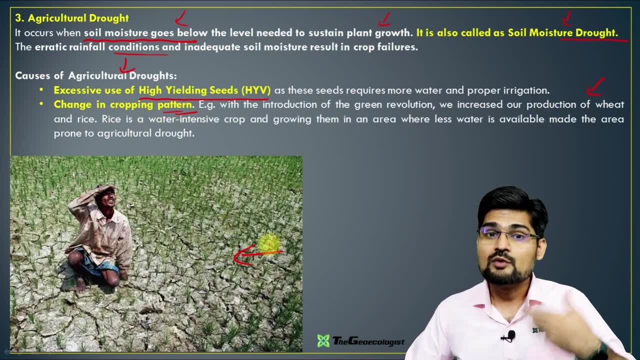 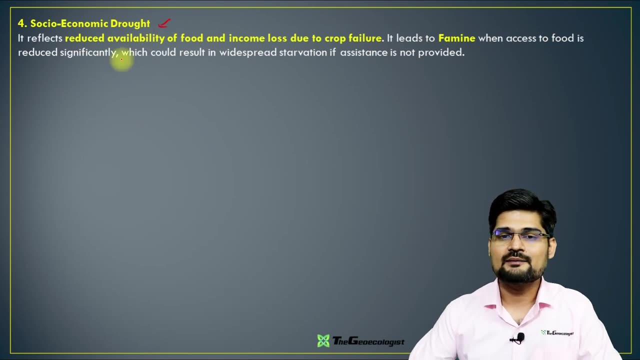 traditional variety going out and modern varieties, which requires more irrigation. we need to look into it again- And then what we have is drip irrigation, dryland farming and other farming, terrace gardening and several other things coming up because of this agricultural drought right Now. if you look into the socio economic drought, the word itself tells us it's a social and economic parameter deciding whether it's drought or not. So it's reduced availability of food. We talked about hunger index, food security right And income. 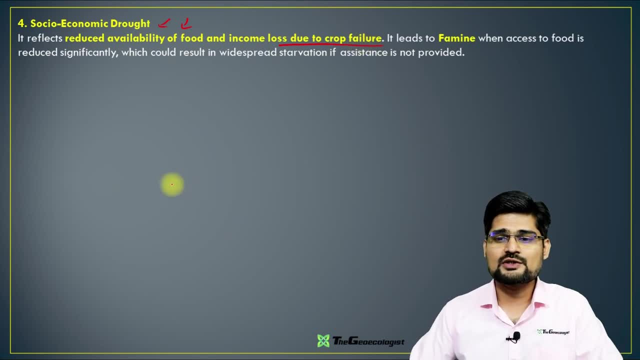 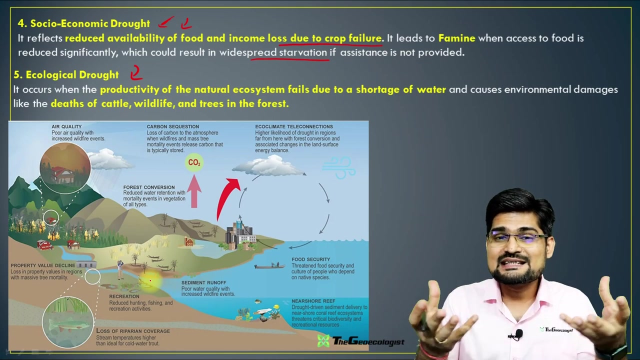 loss due to crop failure. So it's a famine like situation, or you can say a famine arising out of this drought, right, And it's leading to large scale, widespread starvation of people. right. Then comes this ecological drought. So look into this ecological drought Now. ecology is ecosystem, its component. So if they're not functioning properly, then there is this drought. So productivity of natural ecosystem is what is taken into account, where failure due to shortage of water and this particular cycle is. 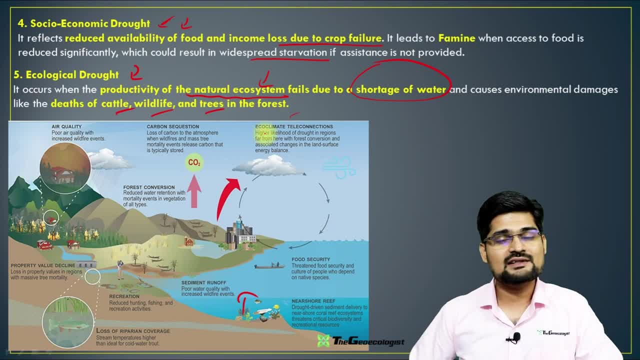 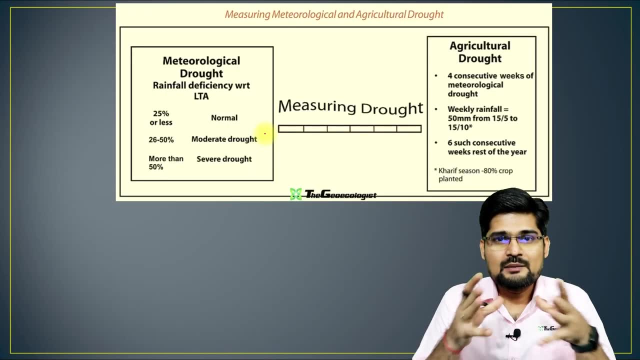 disrupted. So death of cattle, wildlife, trees, forest, everything This is ecological sense. So ecological drought, These are the major types of droughts that you can observe. And now one important thing that IMD also gives us and Ministry of Agriculture also gives us is measuring these meteorological and agricultural drought. What is the significant measurement here? So, meteorological drought, rainfall deficient with respect to long term average LTA. So if it's 25% or less, it's normal, If it's 26 to 50%. 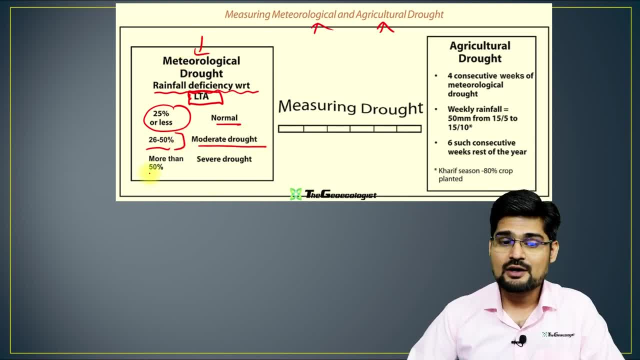 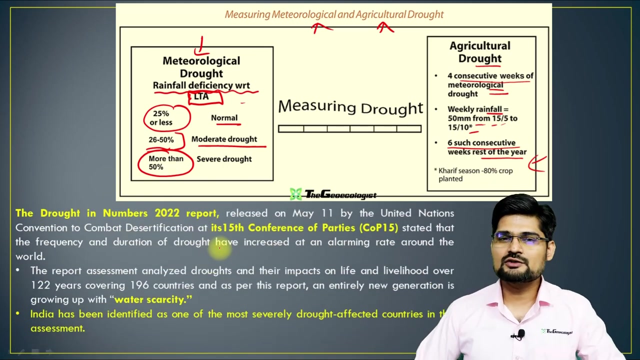 it's moderate drought, But if it's a severe category according to meteorology, what is it? More than 50%, right, Coming to agricultural drought. look at this: Four consecutive weeks of meteorological drought, right, That's the first situation. Then weekly rainfall: 50 millimeter to 15 by 5 into 15 by 10, and six consecutive weeks rest of the year. So then you have this problem of agricultural drought. This is the characteristic. Now look into the situation here through a report. So drought in numbers in 2022: report, if you observe, by United Nations. 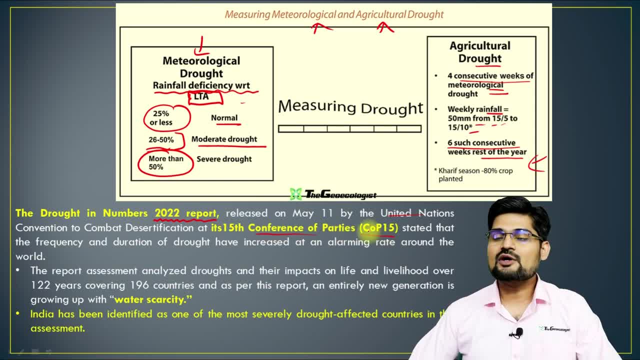 here in 15th Conference of Parties, COP 15,. they talked about combating the desertification right And what you observe? this report gave us the assessment of 196 countries of the world for 122 years of data. This is very significant for your competitive examinations, remember So water. 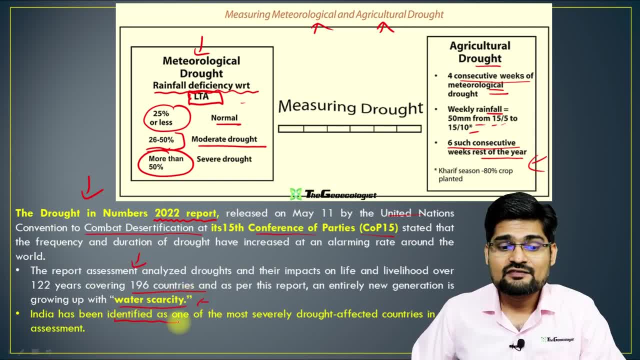 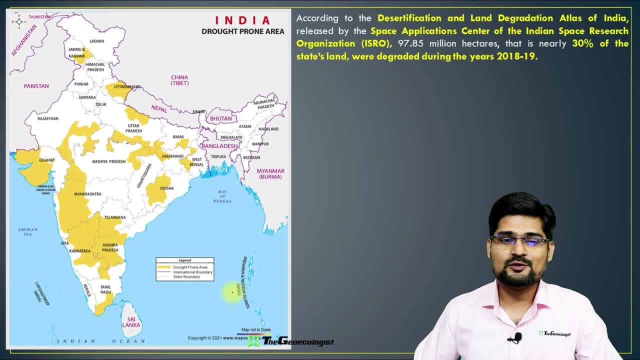 scarcity was observed, and India has been identified as one of the most severely drought affected countries, according to this report as well. So what you observe here in India, the drought areas. I'm sure you have seen this map before as well, in NCRD or many other books as well. So, according 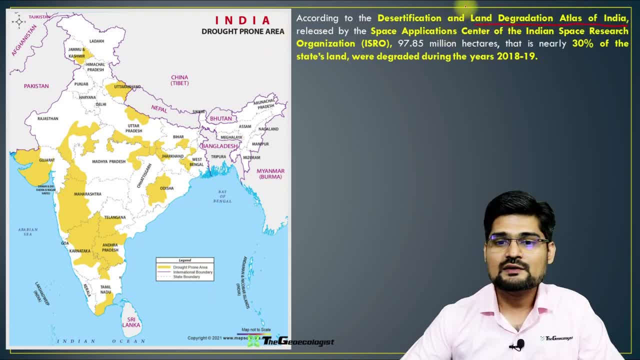 to Desertification and Land Degradation. Atlas of India. Now look into this particular Atlas, Very important, right? It is released by Space Application Center of Indian Space Research Organization, ISRO's work. definitely look into it. Right, It says 97.85 million hectares. 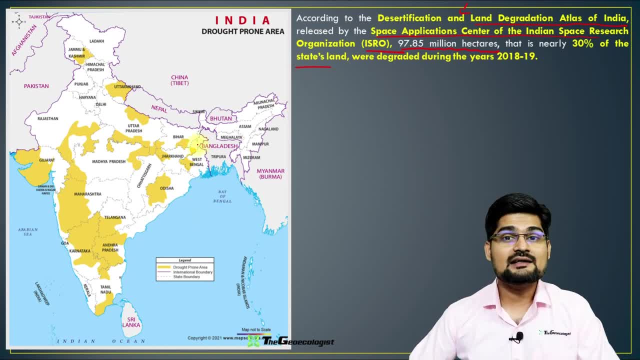 of land. nearly 30% of state's land were degraded during 2018 to 19- only one year. severe drought situation: right. so this is the pockets of drought in India and what you observe here: Uttar Pradesh, Bihar, Jharkhand and West Bengal. these four states are the major ones where rice is being produced. 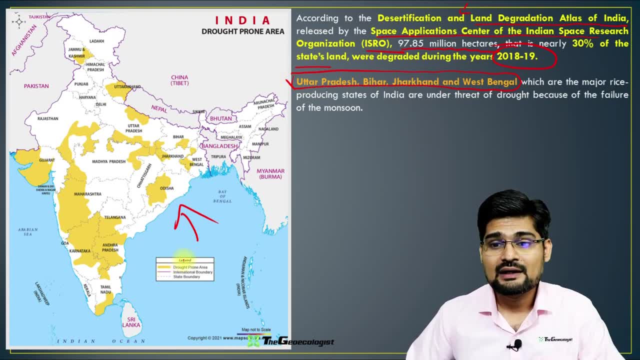 and remember, rice is intensively water-based crop and that's where the threat is. the problem is right. looking into drought prone areas again, the districts nearly comprise one-sixth of this country. the areas receive an annual rainfall of around 60 centimeter or less. and again looking 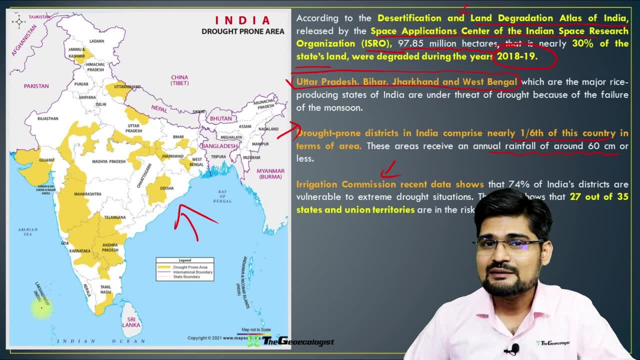 into the further data. irrigation commission. the recent data by irrigation commission tells us 74 percent of India's districts are vulnerable to extreme drought, and that's where disastrous situation is. if vulnerability is more, remember, our resilience is less and that would lead us to disastrous situation. so 27 out of 35 states and UTs in India are under high risk zone, especially. 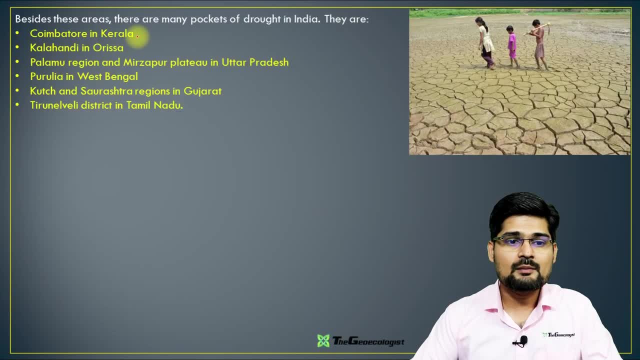 to drought. now look into the other pockets. so Coimbatore in Kerala, Kalahandi, very famous- in Odisha, you Palamu region and Mirzapur in Uttar Pradesh, Purulia, West Bengal, Kachan, Saurashtra in Gujarat and Tirunaiveli district in Tamil Nadu. this is the picture that you represent here, right? so what? 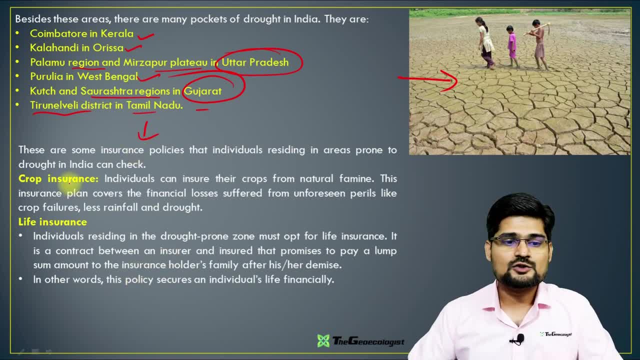 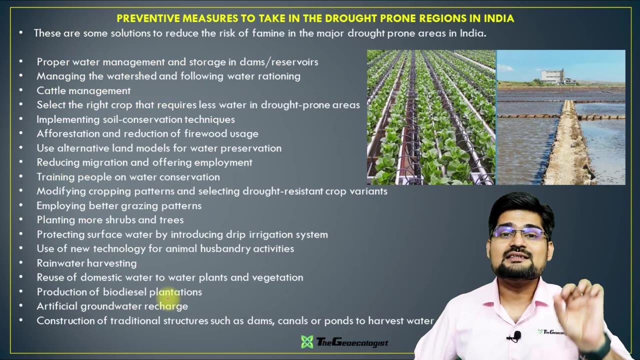 you observe, there are certain insurance policies coming into. so crop insurance, life insurance and all these policies are out there, but still the problem is there. not everybody is able to look into these insurance policies, not everybody is able to get it. but definitely we need to work out on ground level as well. so there are certain preventive measures, right.